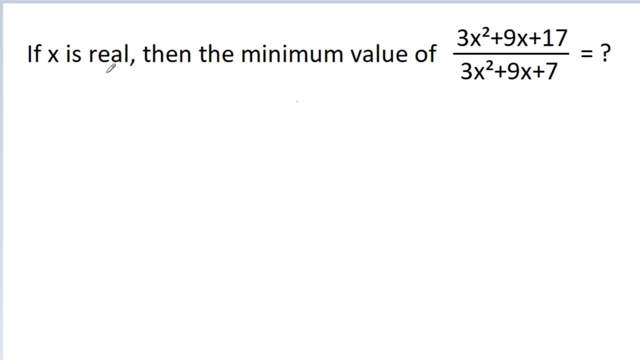 In this video we have given that x is real. then we have to find the minimum value of 3x square plus 9x plus 17 by 3x square plus 9x plus 7.. So, before starting the solution, if this is any function and the range is from 10 to 20,. 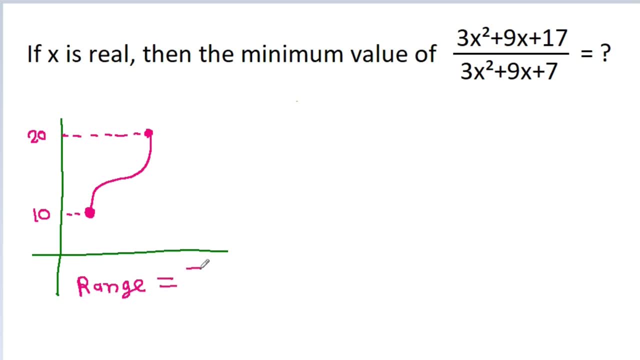 here the range is from 10 to 20,, then what will be the minimum value? Here, minimum value will be equal to 10, and this is the function. and if the range is from open 10 to 20,- here the range is from open 10 to 20,- then what will be the minimum value in this case? 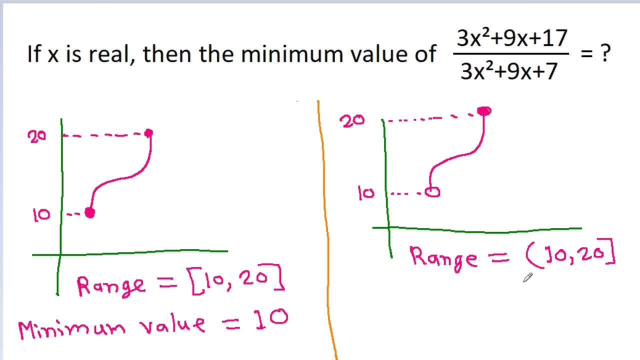 So in this case we cannot find any fixed minimum value, and hence we say that minimum value does not exist. And now we have to find the minimum value of 3x square plus 9x plus 17 by 3x square plus 9x plus 7.. 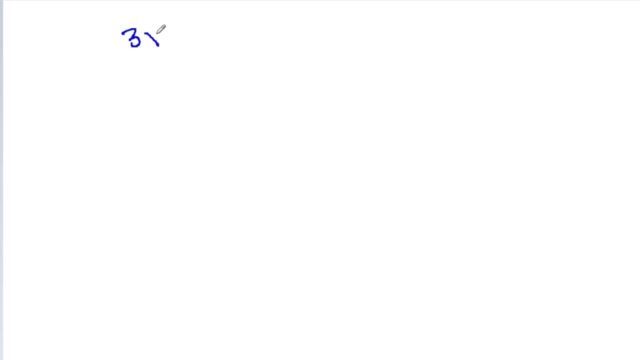 We have to find the minimum value of 3x square plus 9x plus 17 by 3x square plus 9x plus 7.. So if we take this we get: the minimum value of 3x is equal to Y and if we cross multiply. 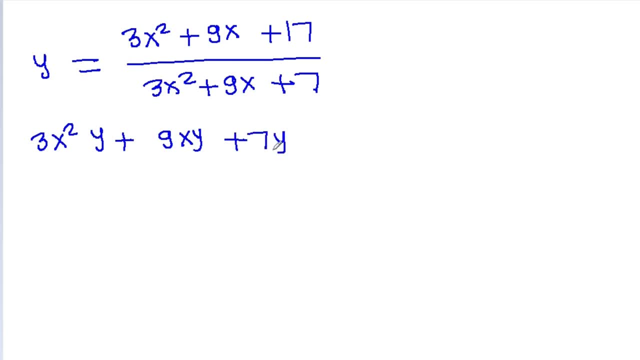 then we get 3x square plus 9x plus 7 is equal to 3 x square plus 9x plus 17.. And its we get 3 x, 2 y plus 9, x, y plus 7 times y, c down to 9x is equal to 3.. 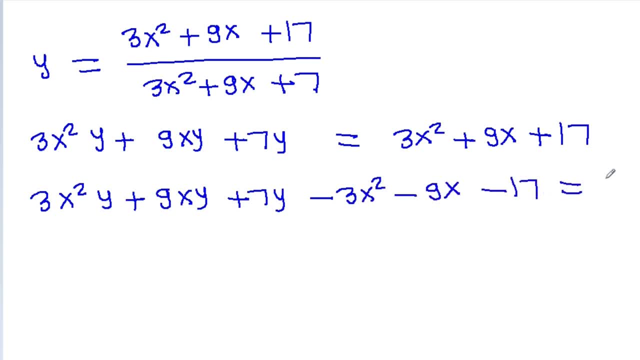 This is 3 x x minus X, squared minus 9 x plus 7.. 9x minus 17 is equal to 0, and if we take 3x square common, then we get y and minus 1 plus. if we take 9x common, then we get y from here and minus 1 from here, plus 7y minus 17 is. 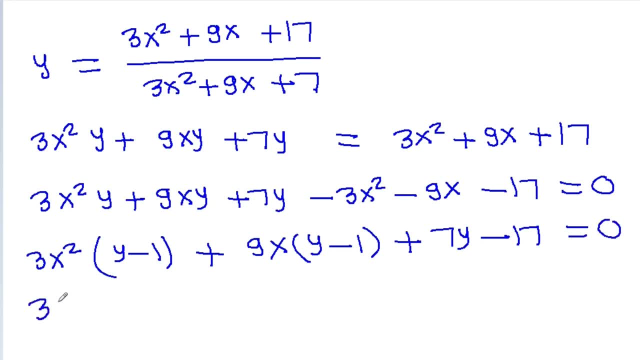 equal to 0 and it is 3y minus 1 x square plus 9. times y minus 1 x, plus 7y minus 17 is equal to 0. so it is a quadratic equation. in x. here it is a times x square plus b, times x plus c. 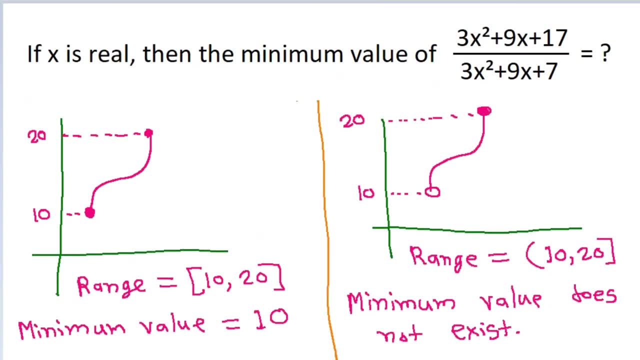 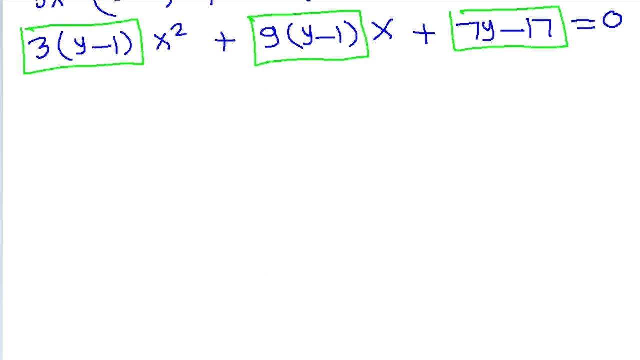 is equal to 0 and we have given x is real. we have given x is real and since x is real, that means d should be greater than or equal to 0 and d is equal to b square minus 4ac and b is 9 times y. 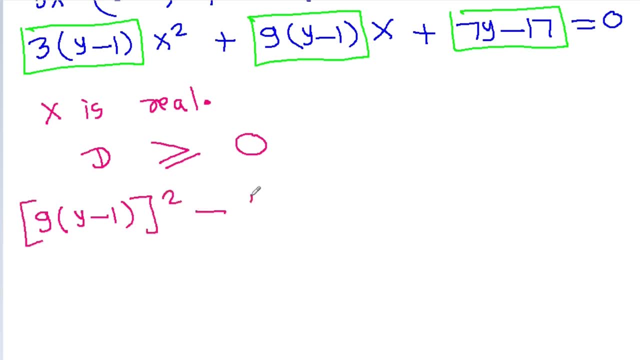 minus 1. square minus 4 times a is 3 times y minus 1, and c is 7y minus 17. it should be greater than or equal to 0 and 9 square is 81 times y minus 1. square minus 4 into 3 is 12 times y minus 1. 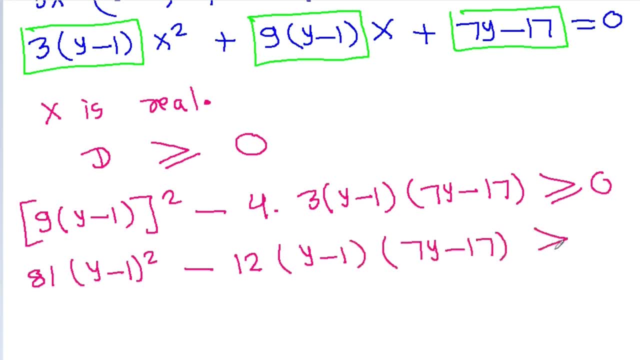 times 7y minus 7y, it should be greater than or equal to 0, and we can take 3 times y minus 1 is common and we will get 27 times y minus 1 minus 4 times 7y minus 17 should be greater than or equal. 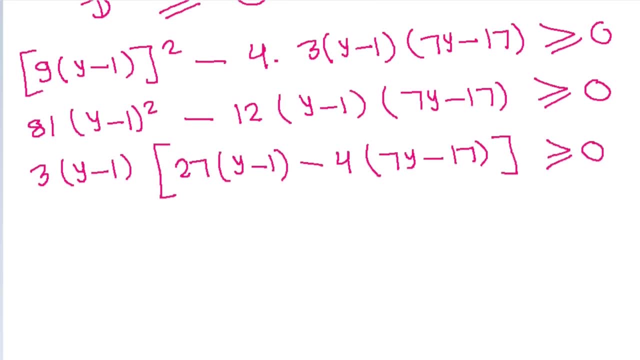 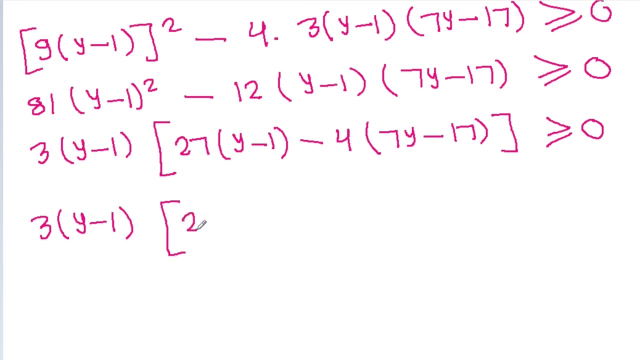 to 0 and it is 3 times y minus 1 and it is 27y minus 27 and minus 4 times 7y is minus 28y and minus 4 times minus 17 is plus 68. it should be greater than or equal to 0, and. 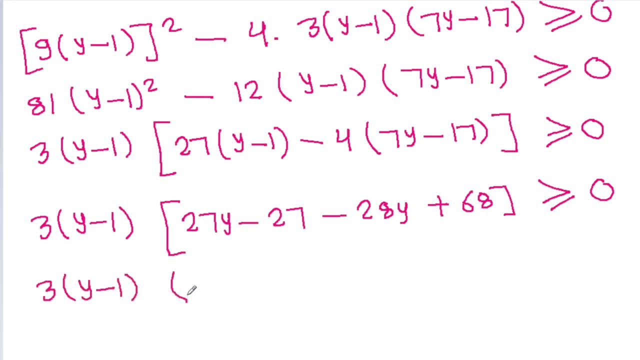 it is 3 times y minus 1 times 27y minus 28y is minus y, and 68 minus 27 is plus 41. it should be greater than or equal to 0, and if we multiply by minus 1, then we get 3 times y minus 1 times. 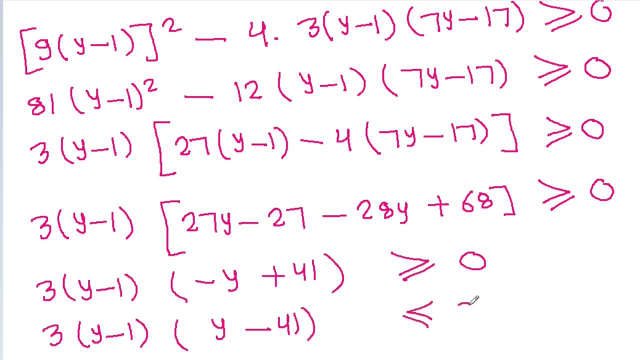 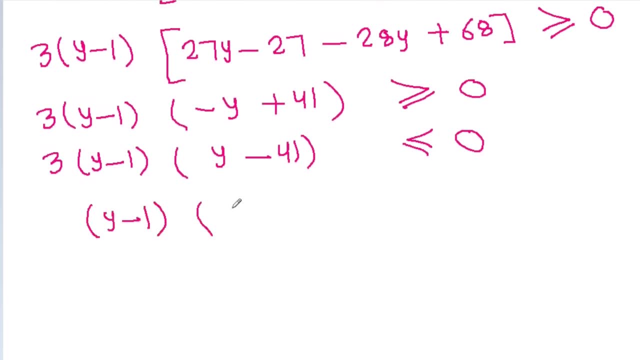 y minus 41, it should be less than or equal to 0.. and it is y minus 1 times y minus 41, it should be less than or equal to 0. so this is 1 and this is 41, and by wavy method this is positive, negative and positive. so y is less than or. 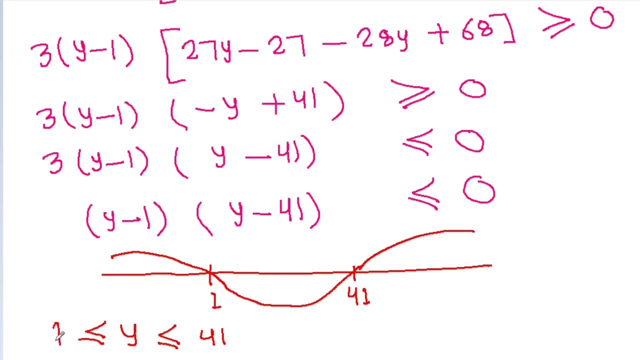 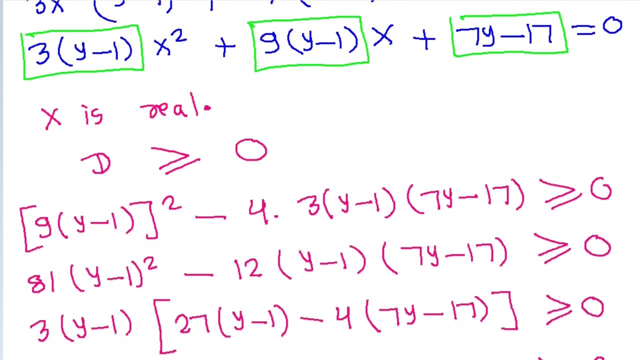 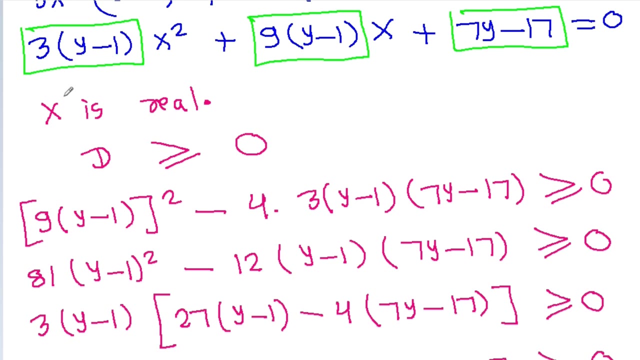 equal to 41.. and greater than or equal to 1, and we have given that x is real. but when y is equal to 1, then coefficient of x square will be 0 and coefficient of x will be also 0, so there is no x left in this equation when y is equal to 1.. 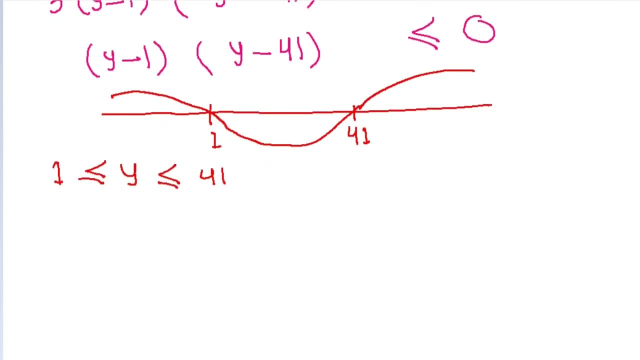 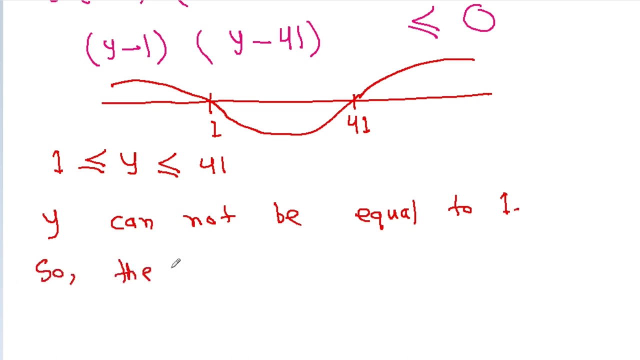 that means y cannot be equal to 1. so the range of y is from open 1 to 41, and hence y is from open 1 to 41.. and hence y is equal to 1. so there is no x left in this equation when y is equal to.